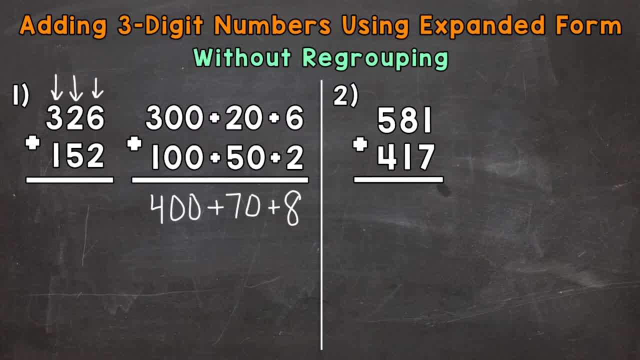 Now that we have that, we can put it together for our final answer: An eight in the ones place, a seven in the tens place and a four in the hundreds place. So eight in the ones place, an eight with a value of eight, a seven in the tens place because we need the value of 70 there. 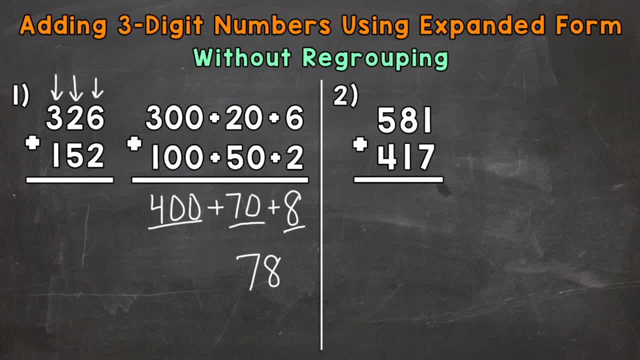 and then a four in the hundreds place, because that four has a value of 400. So 400 plus 70 plus eight gives us an answer of 478.. Now if we were to solve this using the problem to the left, without expanded form, we would get the same thing: Six plus two. 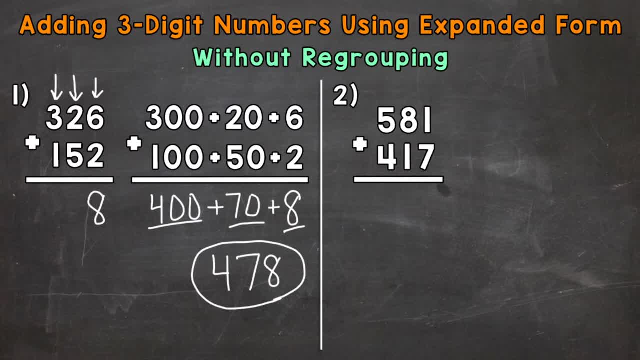 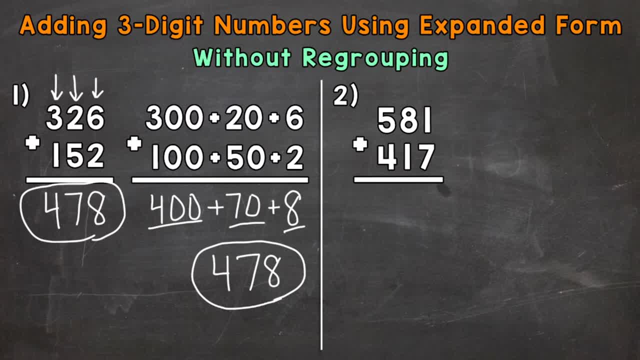 five percent omit of from or by 특히. So if you want different numbers, you can also add in Scott. And then let's take a quick look at the math method. OK, so a heap contains what we had in eight diferente information. We never look at a hundred of pieces of paper, But what? 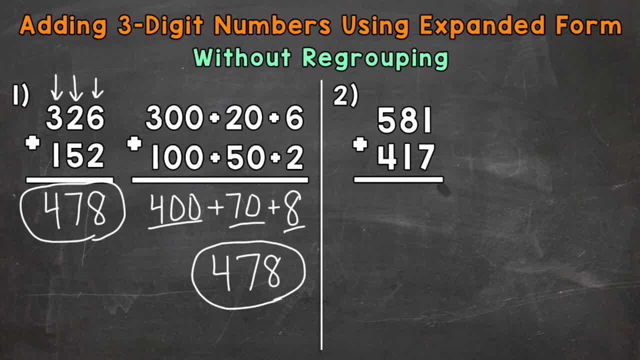 we have these numbers for is the math method that goes along with depending on an blamed losses function? Alright, so that's how we do the math of editing information, the way that Ed Ào advises us. But note: Female and male do equally well. to all we add in the initial: 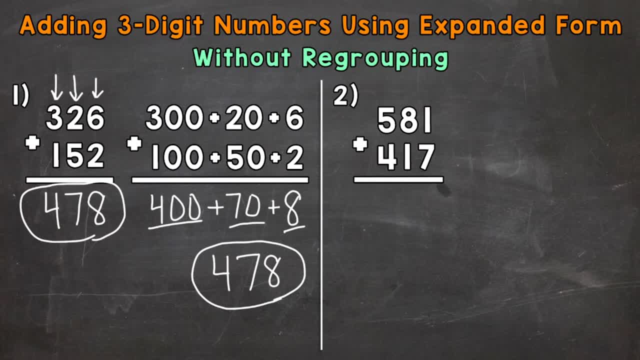 581 plus 417. so for this one we're going to need to put these numbers into expanded form: 581. we will do first. so we have a 5 in the hundreds place that 5 represents 5 groups of 100 and has a value of 500, plus an 8 in the tens place that 8 represents 8 groups of 10. 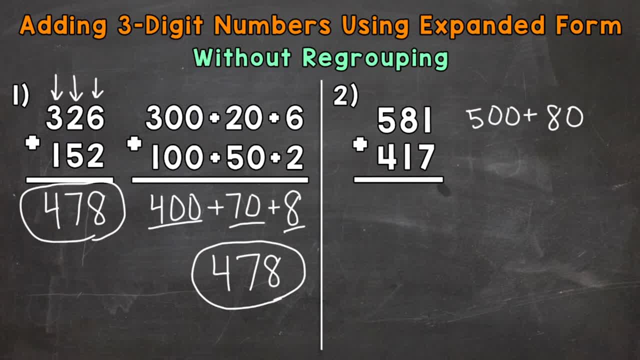 so a value of 80 plus a 1 in the ones place, so that represents 1, 1 which has a value of 1. let's do 417, so a 4 in the hundreds place, so that 4 has a value of 400.